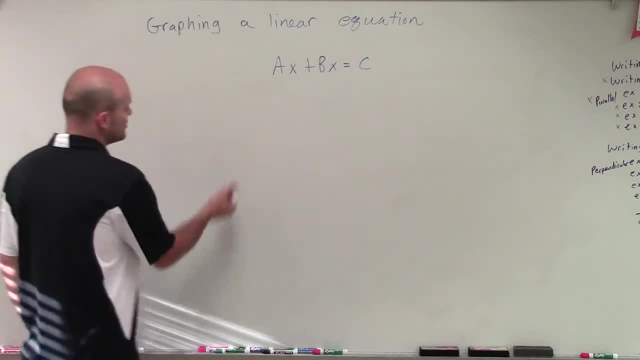 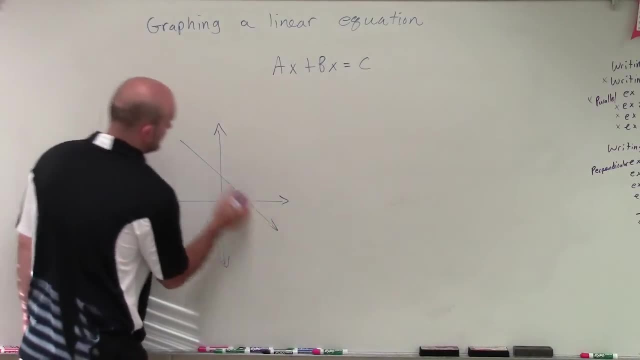 x, Just graphing it by using our x and y-intercepts. So the main important thing I just want you to look at is if we were looking at a graph, all right, and let's just say we have a linear graph, We know that this linear graph is going to have an x and a y-intercept And it's very 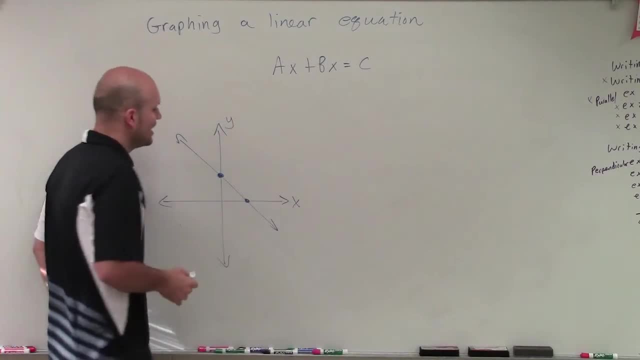 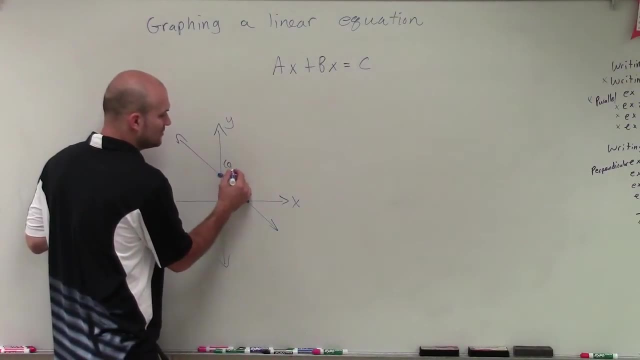 very important for us to understand that. here's my y-axis and here's my x-axis. At this point where this graph crosses the y-axis, we know that the x value is going to be equal to 0, but we're going to have a y value. 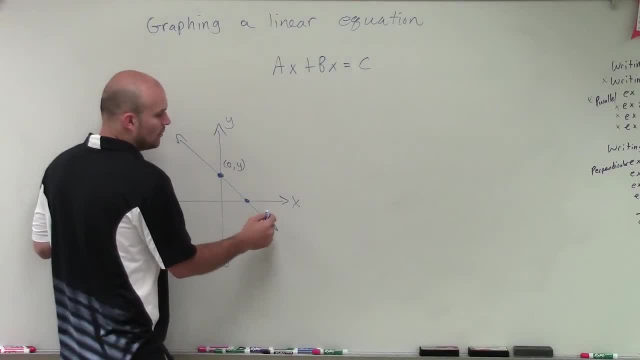 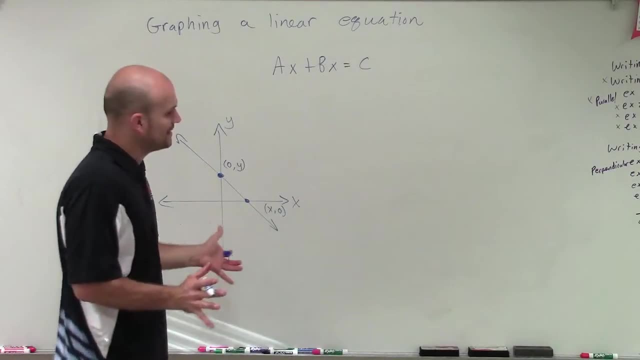 And in the same thing, when we're looking at the x-intercept, we know that we're going to have an x value, but our y value is going to be 0. And that's very, very important, because when I'm going to be graphing using my x and y-intercepts, what I'm going to do, 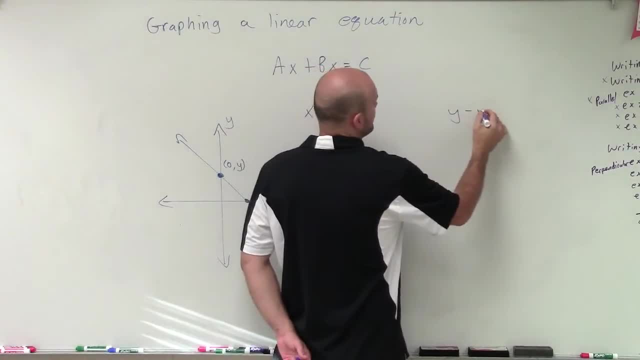 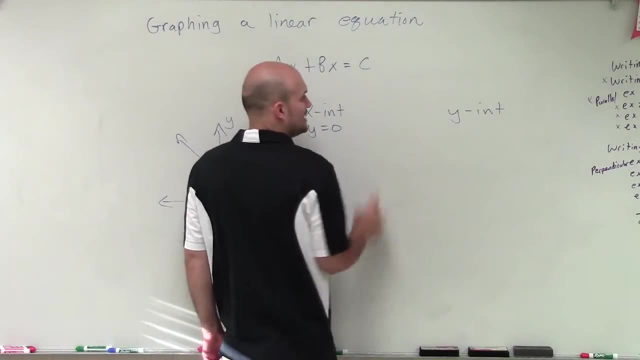 is. I'm going to want to determine what the x-intercept is and what the y-intercept is, And what I notice about the x-intercept is that y equals 0. And for the x-intercept, x equals 0. Right, 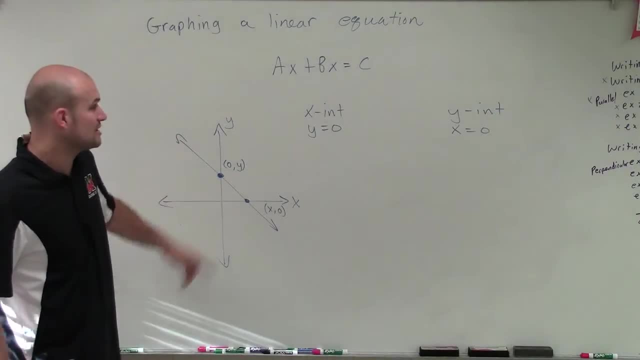 When you look at the x-intercept or the y-intercept, you notice that the x value is equal to 0. And that's very important, because what we're going to do is we're going to- oh, I'm sorry- ax plus by equals c. 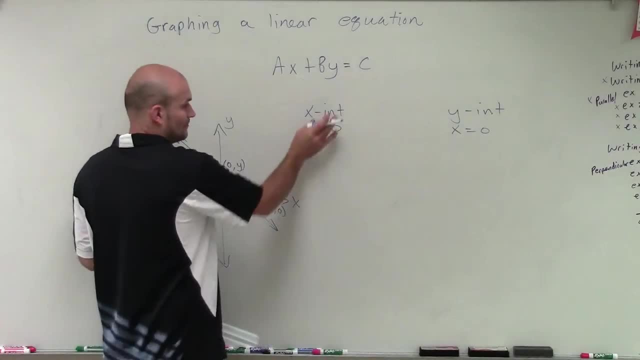 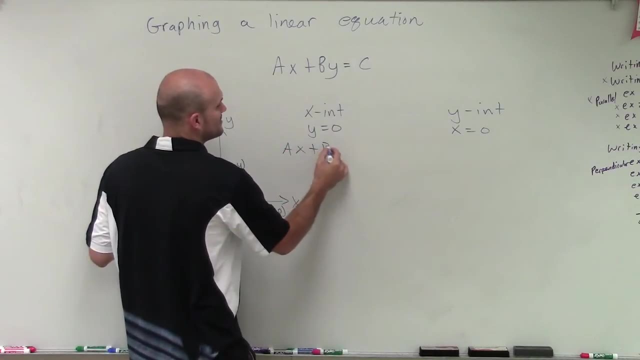 So that's going to be very important, because what we're going to do is, if I know, y equals 0 for the x-intercept. I'm going to plug 0 into this equation, So I'd have ax plus b times 0 equals c. 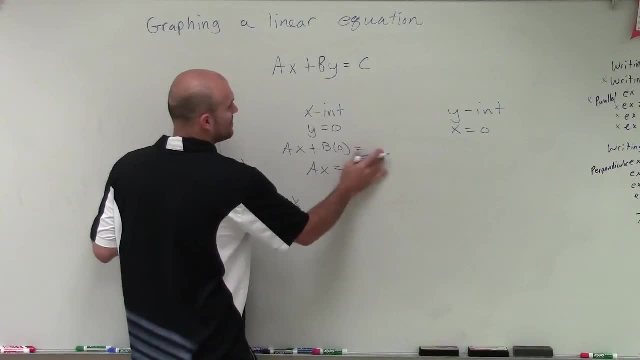 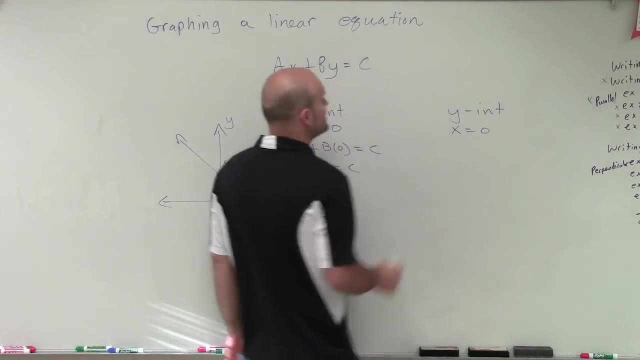 So therefore, ax equals c, And then what I can do is, depending on what values I have for a and c, I'll be able to solve for x The same exact thing. now, when x equals 0, I'm going to plug a 0 in for the x. 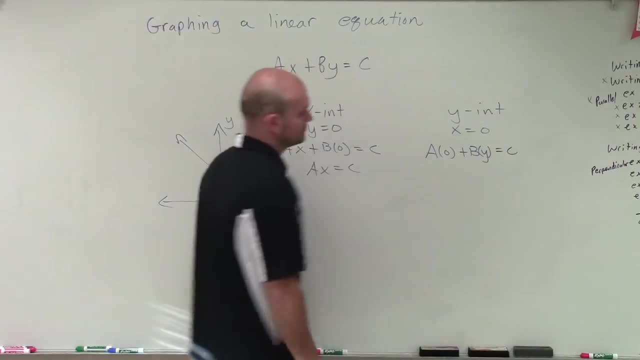 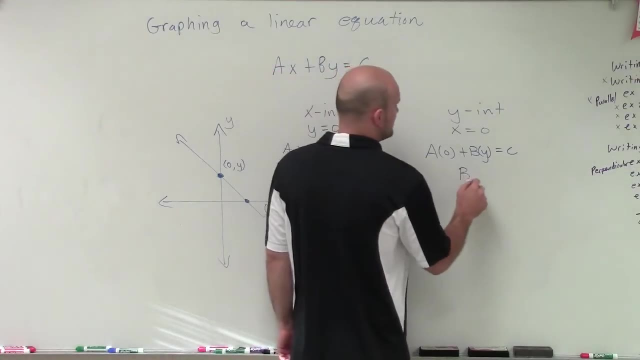 Rosa, please report to the main office. Rosa, please report to the main office. I guess I can't control everything. So a times 0 plus by equals c. Therefore, I'll just have b times y equals c, Depending on what values I have for b.